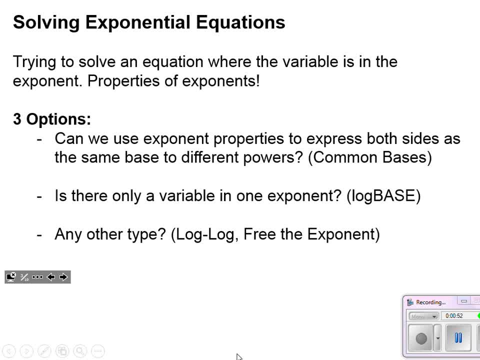 in order to help us rewrite and make the overall equation easier to work with, We've got three options, So anytime we're dealing with an exponential equation, we want to kind of look in this order because we have methods of solving each one. But if we can manage to find one of these steps that's higher on the list. 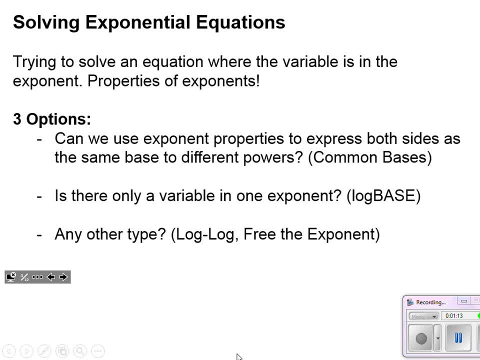 it's going to be an easier problem to deal with. The first and easiest method, if it works, is: can we use our properties of exponents to rewrite the equation so that we have both sides of the equation as the same base raised to different powers? 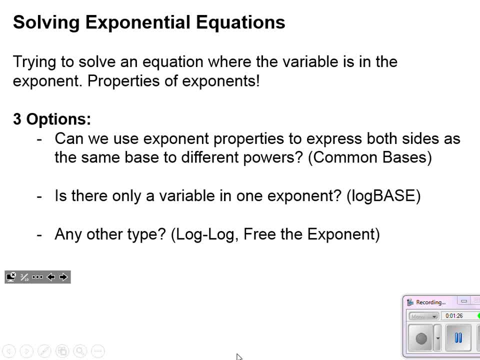 This is called the common base method and it really makes an easy problem Out of a very difficult one. So naturally we want to look for this one first, This one's especially. you know, it should be something that we can recognize pretty quickly. make a couple tests in our calculator maybe. 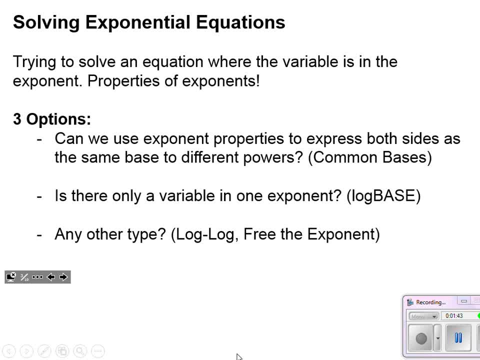 But we'll pretty quickly decide whether or not we can use that method. Secondly, is there only a variable in one exponent, So we can't use common bases. Maybe that doesn't work out If there's only a variable in one exponent. everything else is just a number or something else that we can work with. 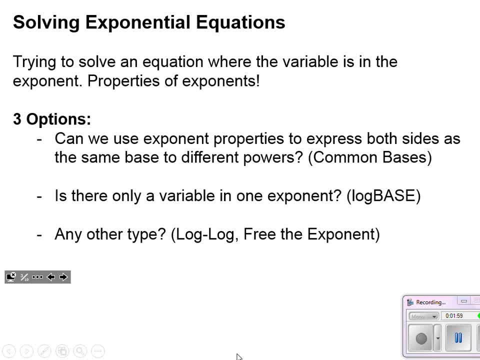 that's when we use log-based. This is a feature on most newer calculators and it allows us to use the idea that Logarithms and exponents are inverses of one another in order to get to that exponent. so that's our next fastest method. If we couldn't use common bases, then log base is the way to go. 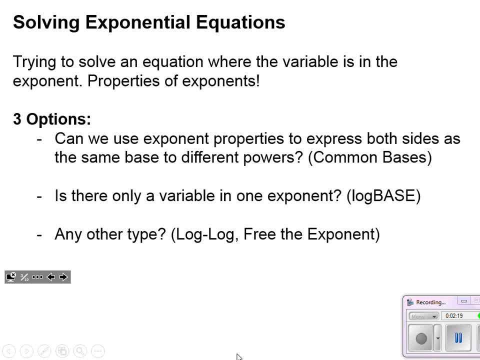 Then lastly, if there is any other type of exponential equation. maybe we have different bases but we have variables on both sides. Maybe it's a complicated problem involved in learning a certain problem solving, like compound interest or something we're trying to solve for a variable in the 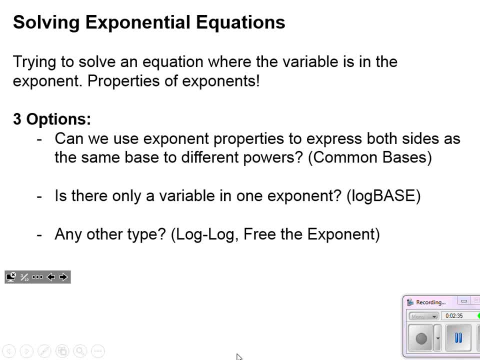 exponent, then our best bet is to use what I call log log, free the exponent And what this means. when I say log log, we can annotate our notes a little bit here. We're going to take the natural log of both sides. 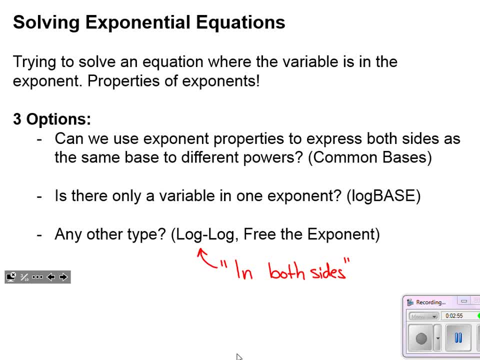 Because one of our properties, let's say we natural log one side of the equation and we have the natural log of what was three to the x minus four power. If I take the natural log of that side of the equation, I'm allowed to free that exponent and it becomes just a regular. 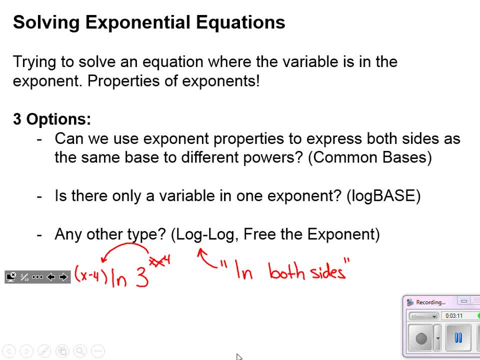 term out in front that we can solve for In the calculator we can easily type in natural log three. So it takes that exponent and makes it something that we can work with. So that's our last resort option. It's typically a little bit more writing, but it will solve just. 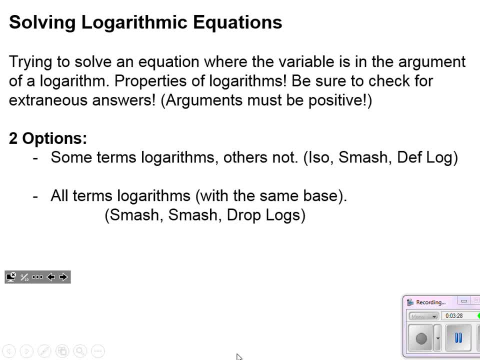 about any other type of problem. So that's our last resort option. It's typically a little bit more writing, but it will solve just of exponential equation, All right. what about logarithmic equations? Well, we covered all those properties that we had in 6.5, and we can bet that we're going to use 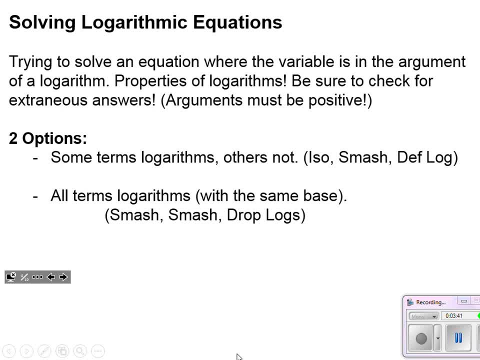 quite a bit of them, as well as the definitions of a logarithm. You know the base is the perfect exponent that will turn the base into the argument of that logarithm. Now one thing: we're going to have to be sure that we check our answers because it is possible that 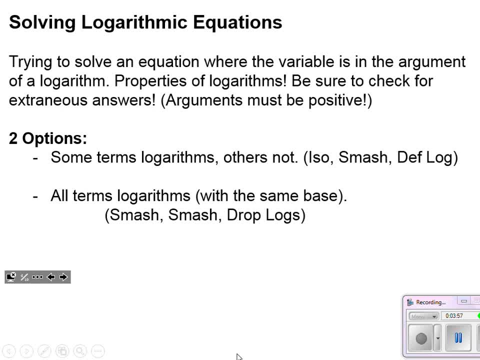 we will get more than one solution And we're going to have to be sure that we check our answers, because it is possible that we will get more than one solution. And when I get more than one solution, I just want to make sure that when I plug it back into the original. 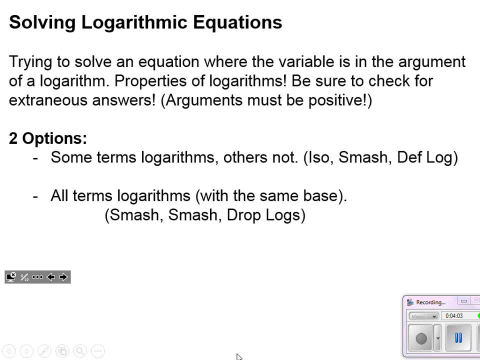 problem. it doesn't make any negative arguments in that logarithmic equation. If it does so anywhere, it's not an acceptable answer. So we can have extra answers there. We want to be sure we're checking for those. We've got two options for solving logarithmic equations. 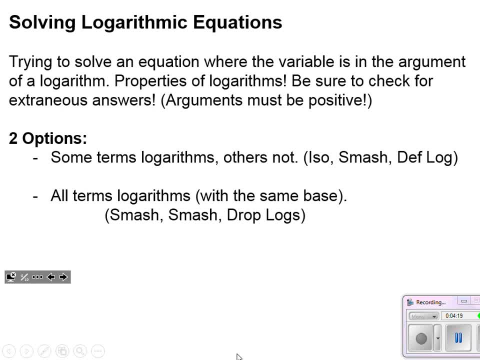 The first one. if I have some terms in the equation that are logarithms, others that are not, I call that ISO SMASH DEFLOG. We're going to isolate, in other words, logs on one side. We're going to smash, that means condense, to a single log on that one side. 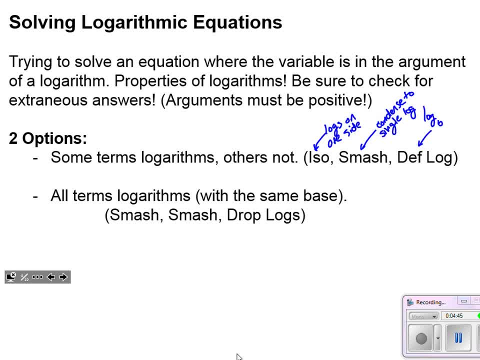 And then the definition of a logarithm says that the base, the logarithm, is that perfect exponent. it is x to get to that power. So b to the x-th equal a. we'll use that to solve the problem, But I think using the having a quick, easy to 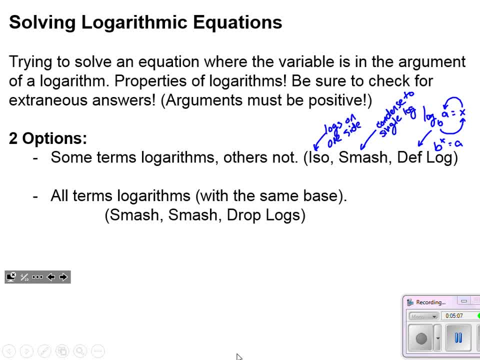 remember kind of a memorable little slogan for this type. isosmash deflog is a nice way of kind of saying: oh okay, I know how to do this, isosmash deflog. It makes it easier to remember. 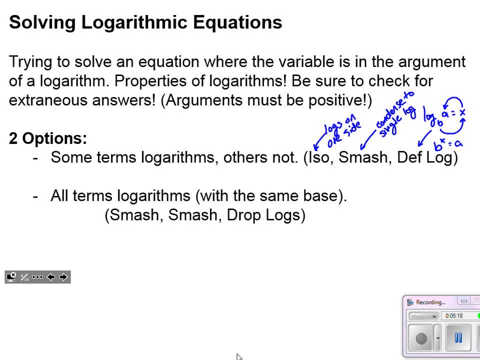 The other option. well, what if some of the term, or, sorry, all of the terms are logarithms and they have to have the same base for this to work? then we're going to take both sides. smash the left side to one log. smash the right side to one log. 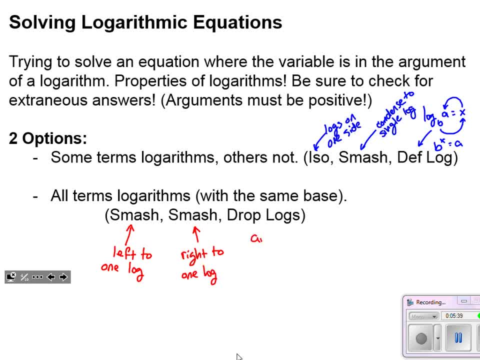 and then we drop the logs entirely and it just becomes argument equals argument, typically a very easy equation. This second option- if we do see an equation that's set up this way- is much, much faster, provided, of course, that we do all of the work with the 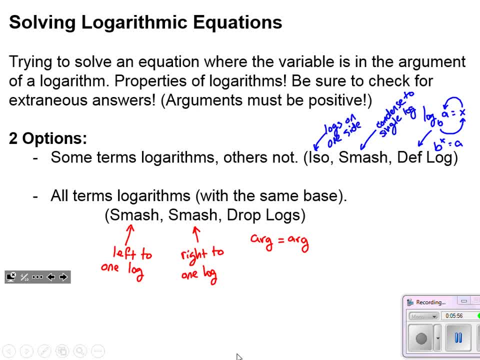 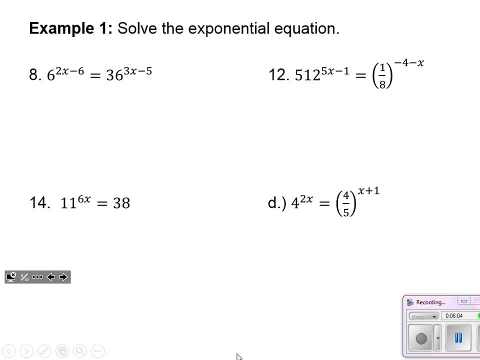 properties to combine all the logs. All right, so we've got quite a bit on our plate and we are going to take some time to learn this, so be patient with it If you need to go back and see how an example was done, please. 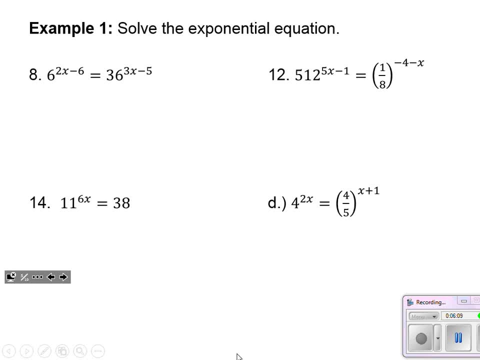 by all means go through and do just that. That's the wonder of YouTube is: you can go and rewatch an example if it didn't make sense the first time. So I hope we take full advantage to understand this fully. This was one topic that, when we had our final exam last year, students struggled with. 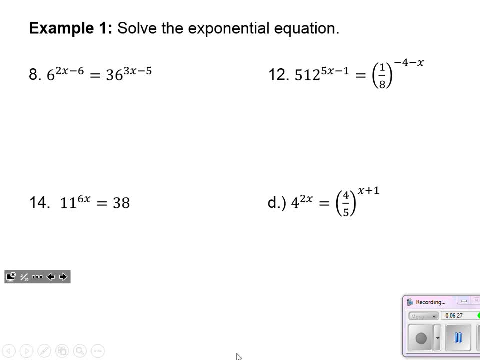 this one. You can save yourself a little bit of heartache later on by investing a little bit of effort right now. So here you can see. we've got four different exponential equations. The variable that we're trying to solve for is in the exponent in each of these problems. Let's take a look at how we can. 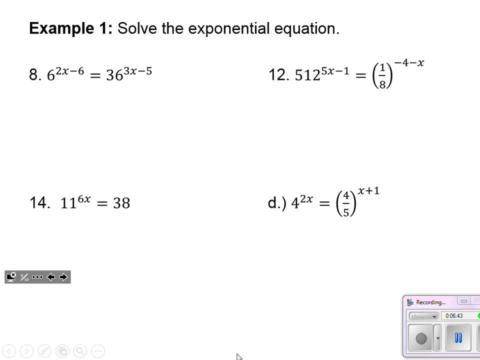 handle each different type. So we'll start off with problem eight here. First I'm going to check and see. can I write: 6 to some power equals 36 to some power. Can I write that as both of those having the same base? 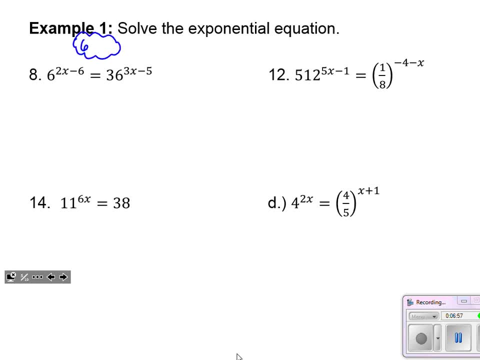 Well, I know, and just give me a second here. I'm going to check and see if I can write: 6 to some power equals 36 to some power. So I'm just kind of thinking up here in my head that 6 to the second equals 36.. Oh well, then I can. 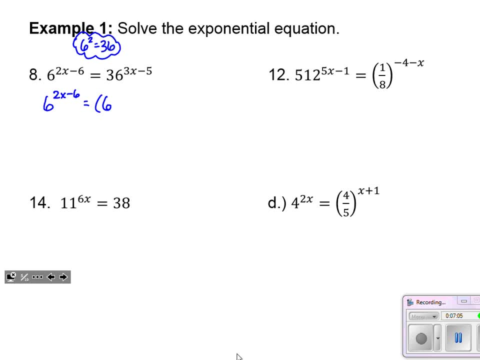 leave the left side alone. but on the right side I can call that 36, 6 to the second. It's just a substitution. But now look at the ultimate base on both sides is a 6.. We've got a common base. 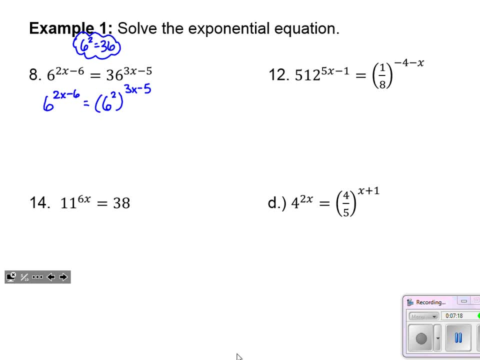 and this is great because this is the easiest way to do that. I just need to know that when I raise a power to another power, I multiply the exponents together, and that requires distributing that power of 2 into that power of 3x minus 5.. Let's see what that does for our 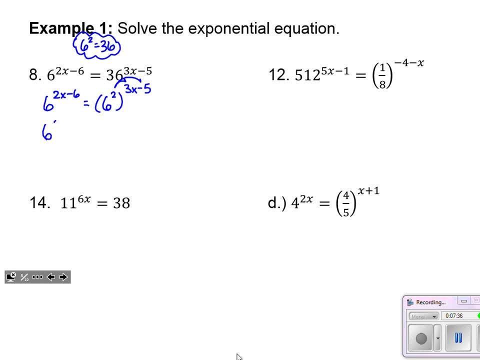 equation. So now I've got 6 to the 2x minus 6 equals 6 to the 6x minus 10.. Because they are both 6 to some power. if those terms are going to be equal, then the exponents have to match. 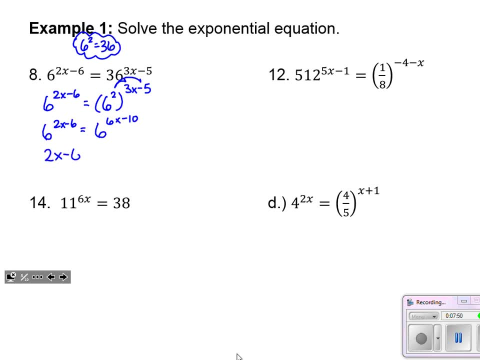 because the bases already match perfectly. All I'm really trying to solve is 2x minus 6 equals 6x minus 10.. Subtract 2x from both sides, add 10 to both sides. I find that x equals 1.. 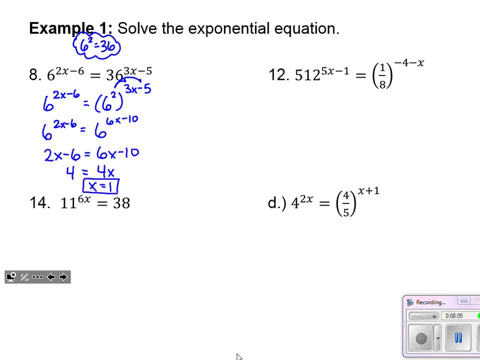 Okay, and I'll go back and plug that in: 6 to the 2 minus 6, that's 6 to the negative first. Does that equal 36 to the negative second? Yes, it does. You know, we can run through a quick check. 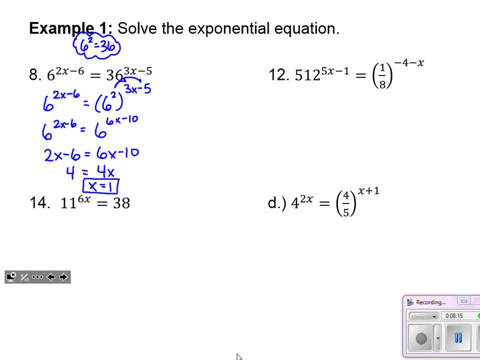 in our calculator if need be. but we very quickly get to the answer if we are able to set up common bases. How about number 12?? Well, 512 and 1 eighth. Well, 1 eighth. anytime I see a 1 over, I know I can use a negative exponent there. 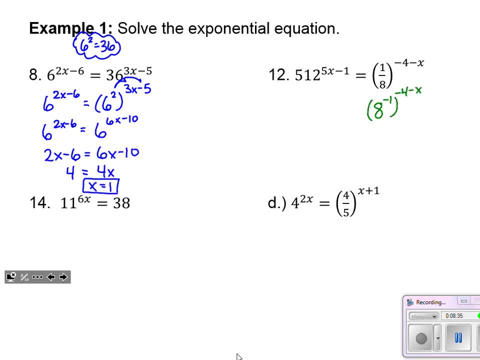 That's 8 to the negative first. Let me just try and rewrite kind of substitute in And 512, maybe I'll test that in the calculator, see if that's 8 to some power. And hey, it's 8 to the third, So I'm able to get a. 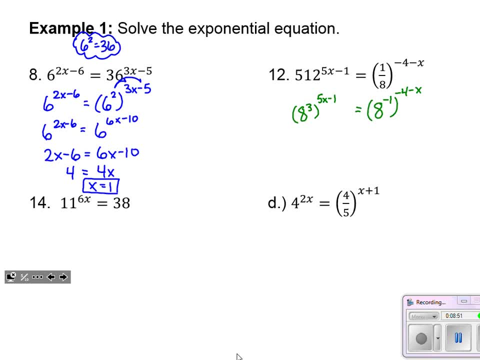 common base, even though it had a negative exponent on the right-hand side. it's still a common base. It still works. It feels like we're cheating the system because it's so easy On both sides. we do have a power to, a power rule to. 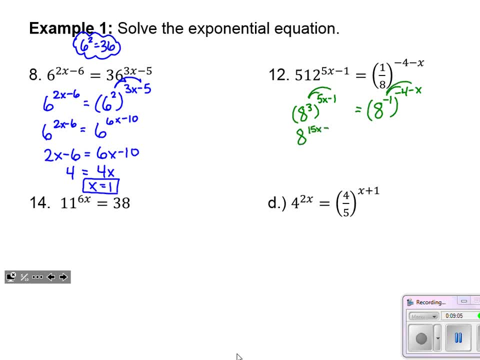 carry out. So I've got 8 to the 15x minus 3 equals 8 to the 4 plus x. Well, if those terms are going to be equal, their bases already match. exponents have to match. So my equation becomes: 15x minus 3 equals 4 plus x. Let's subtract x. 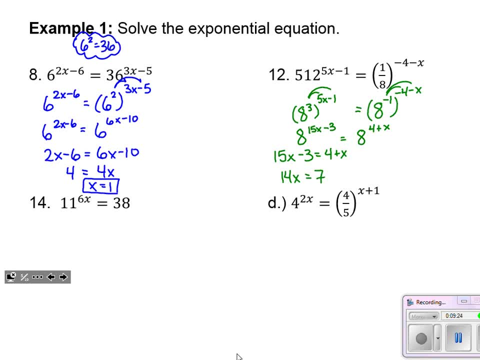 from both sides. add 3 to both sides, X equals 1, half, And it's perfectly fine if we end up with an exponent that's not an integer. Here we've got a fraction. We know that fractional exponents are perfectly acceptable as numbers. they just mean roots. 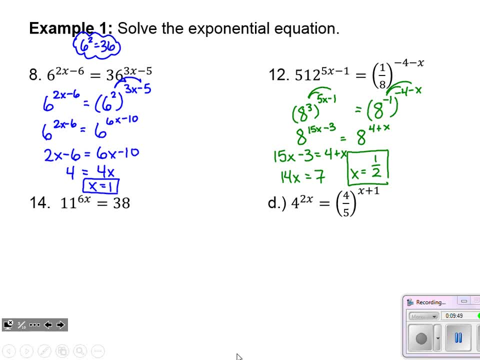 All right. now we get into some more interesting stuff. Those first two: we were fortunate. it may have taken a little bit of time, but we did find common bases and that made the work very easy for us. For number 14, if you look at that- 11 to the 6x, there's no way I can write that 38 on the right as 11 to some power. 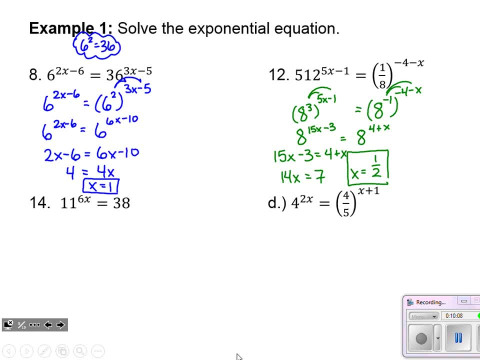 Okay, so I cannot establish common bases. Then I look at: okay, is there only a variable on one side of the equation? And thankfully there is. So now I just need to think of: hey, the only problem is I want to get to this x right here and it's an. 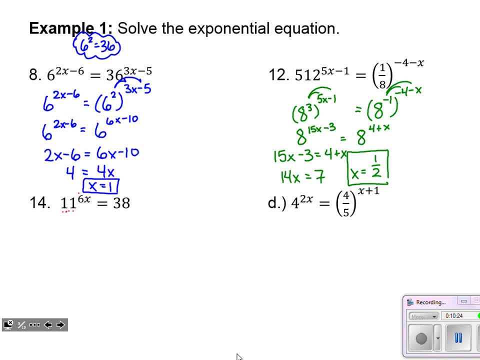 exponent on 11.. So what would cancel out 11 to the 6x? So what would cancel out 11 to the 6x? So what would cancel out 11 to the 6x? Oh, logarithms, Logarithms. So I'm going to take log base 11 of both sides, and that's what we call using the log base method. 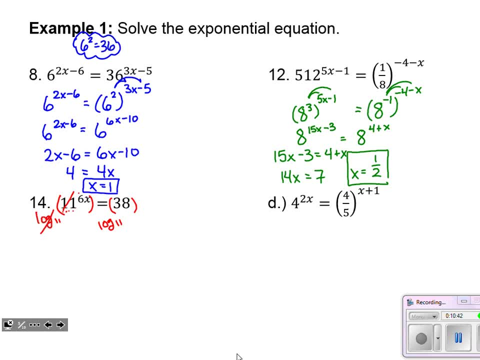 On the left, log base 11 of 11. to some. power is just the power It simplifies away. All we're left with is that 6x. And on the right-hand side I have log base 11 of 38. I couldn't simplify that, but you know what? 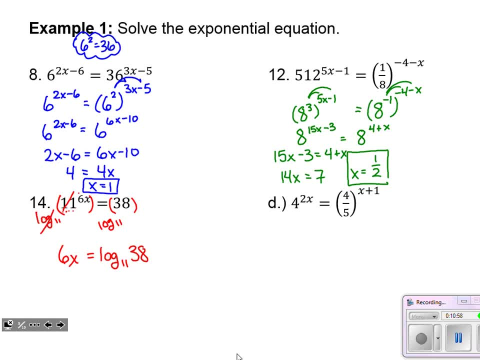 My calculator can sure handle it. So all I need to do in the calculator is type in log base: 11 of 38 divided by 6. And I'll get an answer of type that up really quickly. I get 0.2528.. 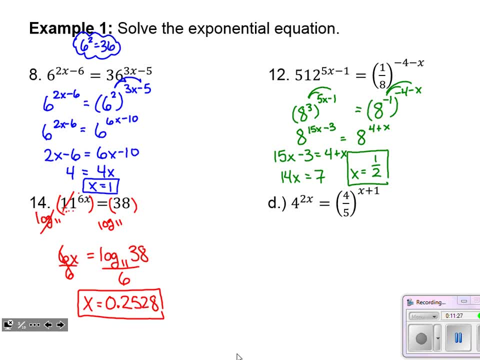 All right, and lastly, let's go about problem D. I guess It's the last example. I kind of added this one off the cuff: Can I get common bases? Well, no, That 4 fifths is really kind of a pain in the posterior. 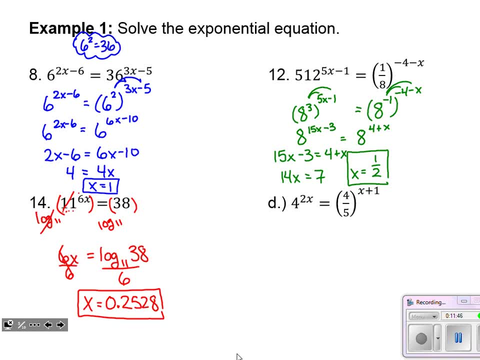 Okay, so common bases are out. Is there a variable in only one of those exponents? No, So log base is out, unfortunately. Luckily, we do have that one last option of log log free the exponent. So I'm going to take the natural log of both sides. 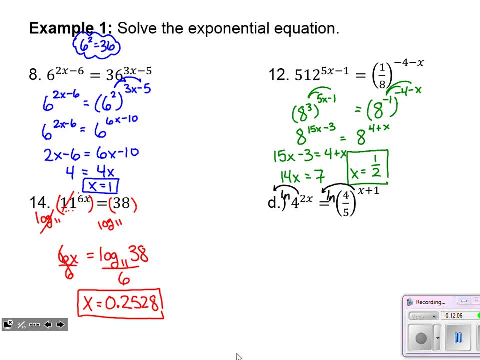 That's going to allow me to free the exponents, And let's see what that sets up. I've got 2x times the natural log of 4 equals x, plus 1 times the natural log of 4. fifths Again. since I'm using natural log, it's an easy type into the calculator. 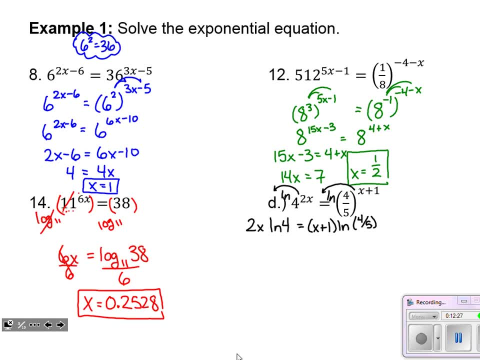 I don't have to go through any menus. It's a key that's right there, ready to use. It's just some decimal, All right. well, what I want to do is I want to group my x terms together, So I need to take this number natural log of 4 fifths and distribute that on the left. 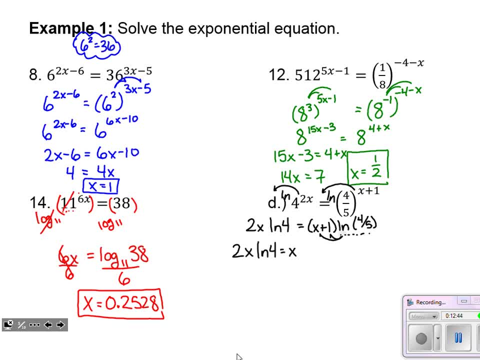 Or on the right, I should say 2x natural log. 4 then equals x natural log of 4 fifths plus 1 times the natural log of 4 fifths. Again, those are just decimals I can get out of the calculator. 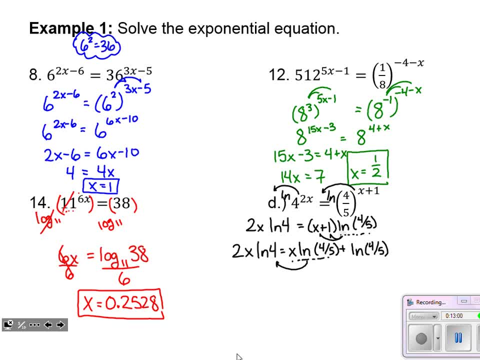 I'm going to subtract over this x term, right, I want to combine like terms. Let's get our x's grouped. So I have 2x natural log 4 minus x natural log of 4 fifths equals natural log of 4 fifths. 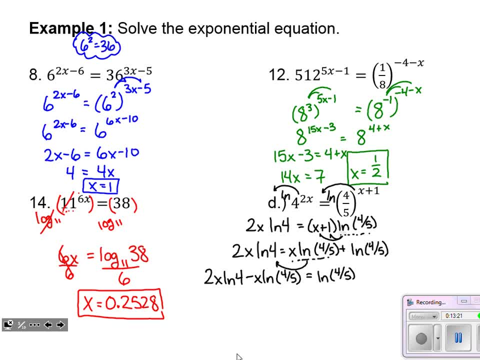 This is why it's our last resort. It does take a little bit more writing, but it's really not too terrible to do Now in order to get 1x to solve, for I can now factor it out as a GCF. 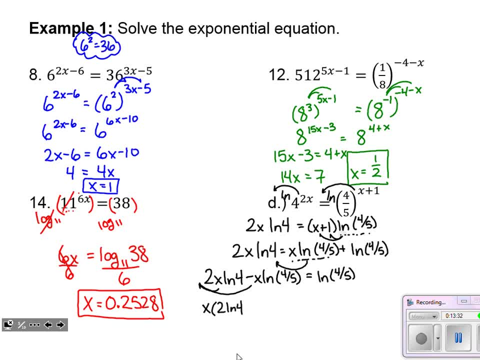 x times 2 natural log. 4 minus natural log of 4 fifths- I've factored it out- Equals the natural log of 4 fifths on the right, And all of this right here can be divided out. It is some number that my calculator can figure out. 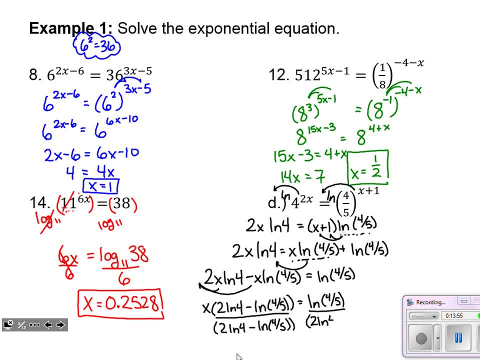 So I'm going to take the time To carefully group everything together, Make sure that it's in the calculator, the right way. All of that cancels out leaving x on the left And once I punch in natural log of 4 fifths divided by that group. 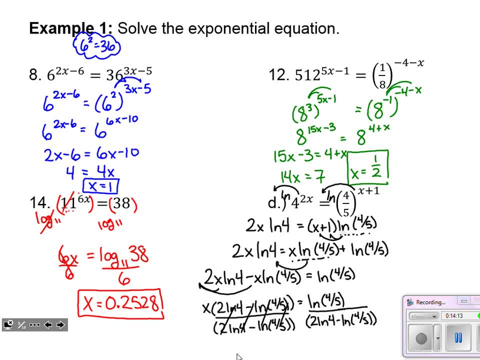 2 natural log 4 minus natural log of 4 fifths Calculator comes out with a solution Negative, .075.. And we can round that to four places. Since it's an exponent, we want to be a little bit more precise than just like rounding to the nearest tenth or something like that. 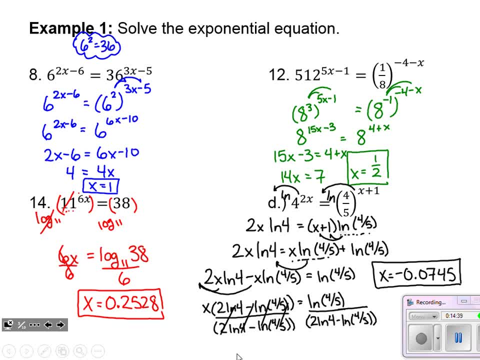 So an answer of negative .1 would be way off. So I typically choose four places when doing exponential equations. So there you've seen the good, the bad and the ugly, The really nice way of using log base and common bases. And then, if that all fails, 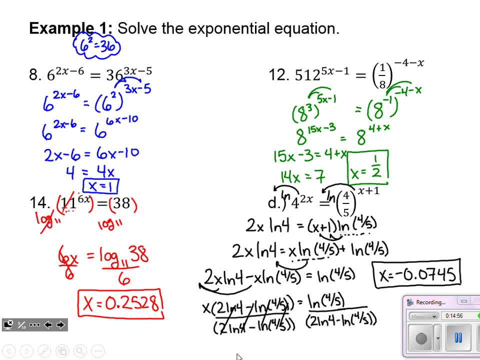 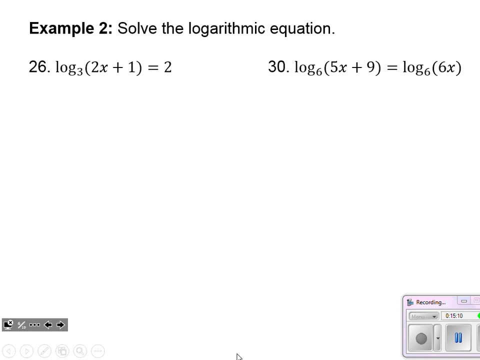 Then we do still have this method that will work every single time By logging both sides and freeing the exponent. All right, moving along, Now we've got logarithmic equations. So for number 26, I just want to see: Okay, do I have some logarithmic terms in that equation, or all logarithmic terms? 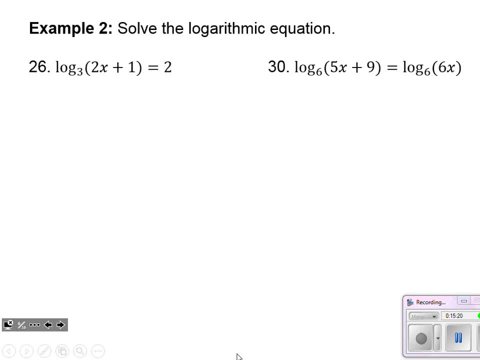 And in 26,. you can see I've got one log and a regular number. Okay, Well, my procedure there- when some of the terms are logarithms, excuse me- is to isolate the logs- that's done, smash them into one logarithm- that's done, and then use the definition of a logarithm. 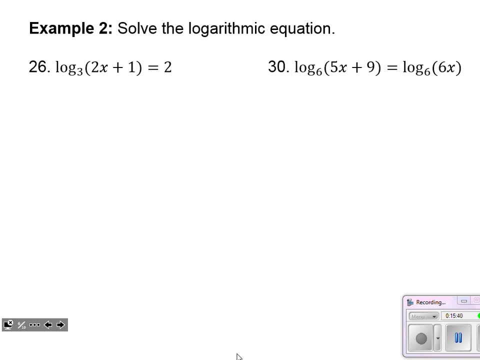 So I really only have to do step three. The definition of a logarithm says that if I have a base of three, the logarithm is: the logarithm equals the perfect exponent to put on that three, to turn it into: oops, not three, 2x plus 1.. 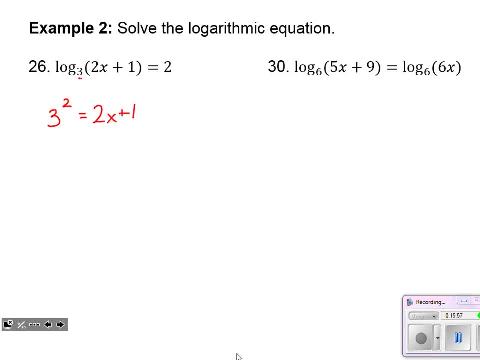 Our argument. Well, I could give this to any freshman in algebra one and they'd be able to solve this. Three to the second is nine. Let's subtract one from both sides, Divide both sides by two and I find x equals four. 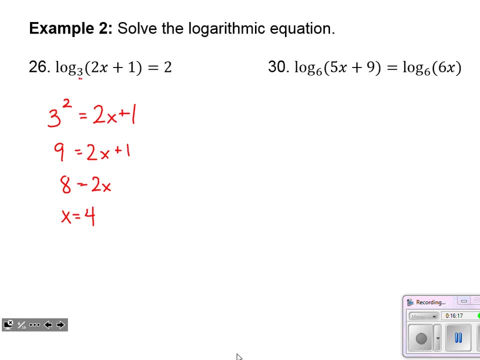 Now I want to double check. Can I plug that in safely without making the argument negative? If I plug in a four, I get 2x4 plus 1.. That's nine. Yep, it works. ISO SMASH DEFLOG. 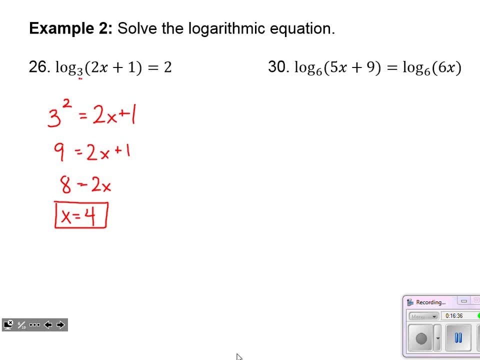 For number 30, okay, do I have all terms that are logarithms or just some of them Here? all the terms in my equation are logarithms and they have the same base. So this is really good. But if one log base six of something equals another log base six of something, then their arguments have to match as well. 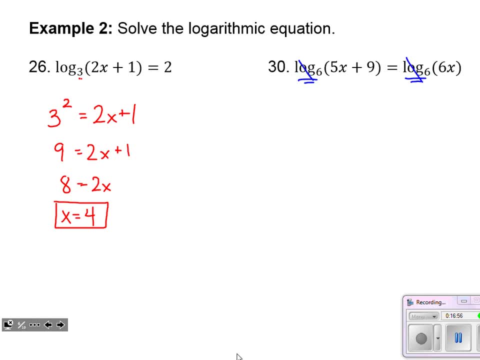 So I can Drop the logarithms out of the problem entirely and I get 5x plus nine equals 6x. We want to be really careful that there aren't any extra, just regular numbers or anything hanging around. This only works if we have one logarithm equaling another logarithm. 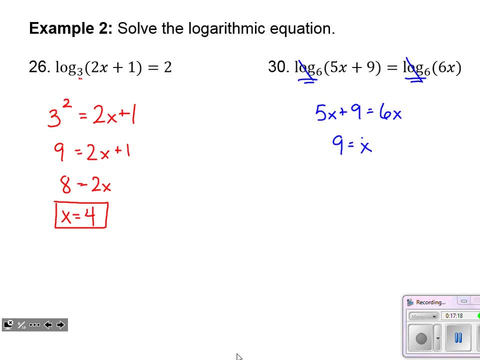 And all I do to solve. subtract 5x from both sides, I get nine equals one, x, x equals nine. Okay, well, let's double check. If I plug a nine back in on the left, I get log base six of 45 plus nine, 54.. 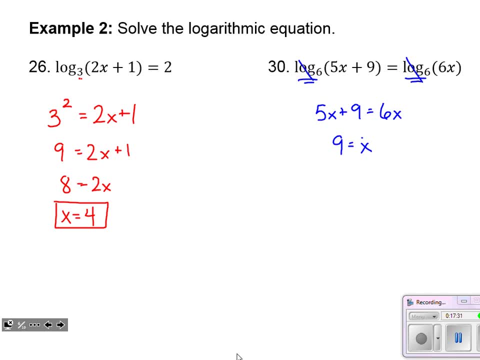 And if I plug nine into the right side, I get log base six of 54.. Yeah, it works. No negative arguments. We get to keep that one, All righty. Next we're going to up the ante a little bit. 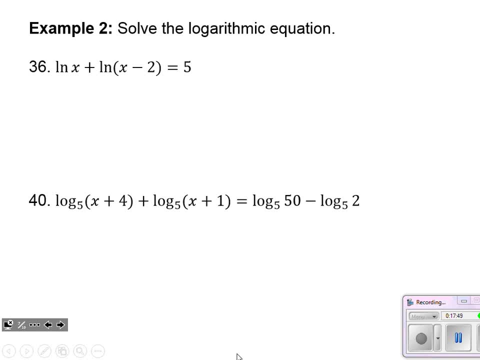 You can see, these equations have gotten a little bit more difficult. For number 36, I've got two logarithms added together. Even though it's ln, that just means a logarithm base, e remember. so we can use all our properties still. 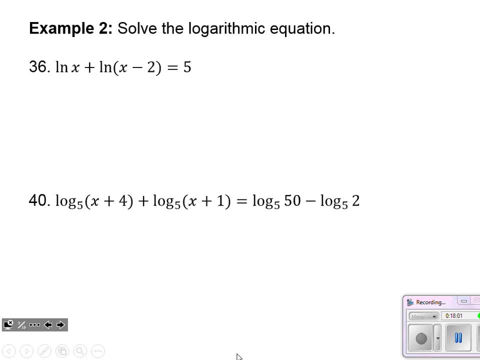 Two logarithms added up equals a regular five. So not all the terms are logarithms, just some of them. So I want to isolate the logarithms. Well, that's already done. They're grouped together on the left. I want to smash the logarithms, condense them into one, and that's where I need to pick up the problem right now. 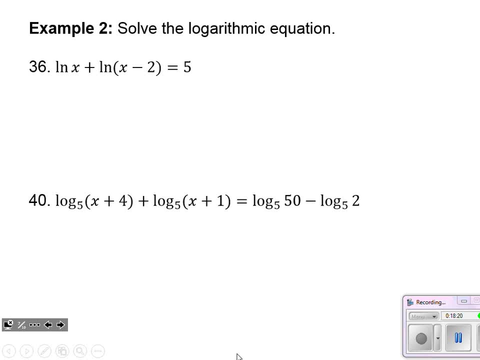 So what I'm going to do is say, okay, I can write this as one. I'm going to write this as a natural logarithm. Since these were added together, it's the same as multiplying their arguments inside a single logarithm, and that's equal to five. okay, 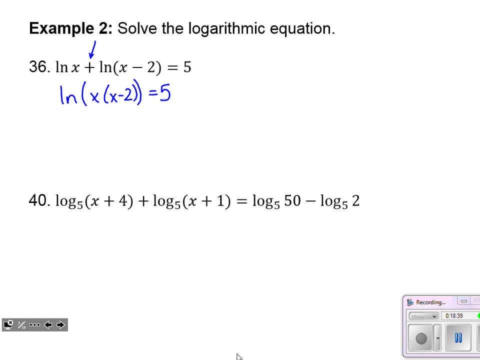 The smashing is done, Isolated. We smashed. Now it's time for death log. So what this statement is telling me- and I can simplify it, call it x squared minus 2x- What this statement is telling me is that, well, I'm going to write this as a natural logarithm. 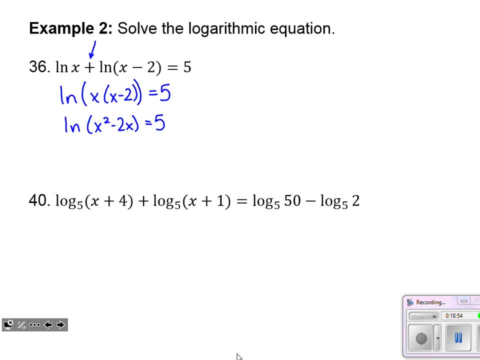 I'm going to write this as a natural logarithm. If I wanted to turn a base of e- and we have to know that that's a base of e in a natural log- if I wanted to turn an e into an x squared minus 2x- the perfect exponent, the logarithm is a 5 to put on that e. 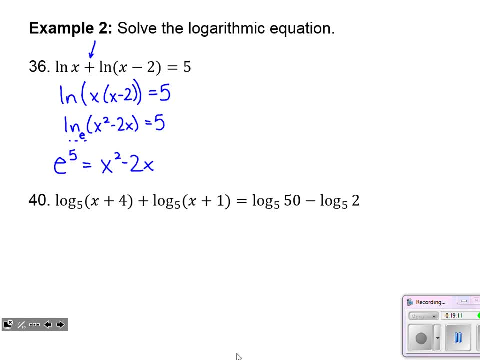 Base of e perfect exponent is 5. to get to x squared minus 2x. Okay, Now it's my hope that you can get to this, no problem, But once we get to this, I'm going to write this as a natural logarithm. 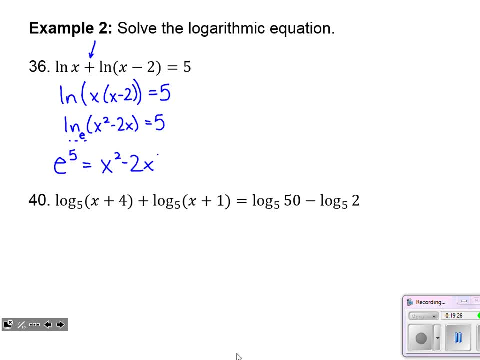 And once we get to this point then it gets kind of tricky to actually find out. you know we're not done solving yet. We want x equals something. How do I solve something like that? Well, it sort of looks like a trinomial. 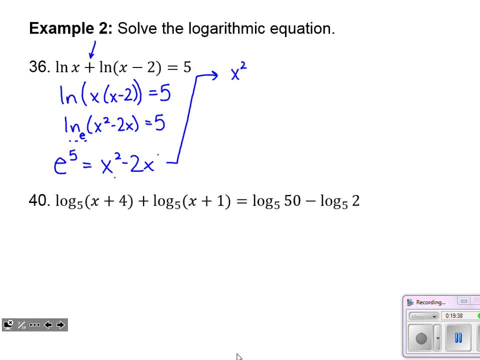 And when we have a trinomial we want to get it set up equal to zero. Remember all that lovely work from chapters two, three and four. So I'm going to subtract over e to the fifth And then we can use quadratic formula. 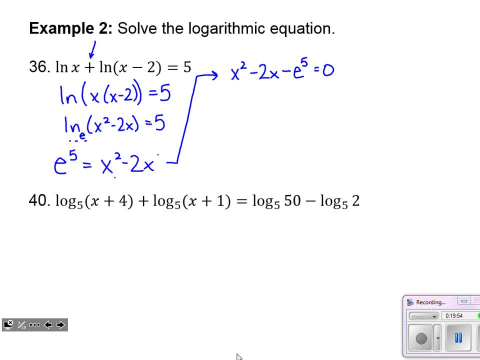 E to the fifth is just a number. So to find my solutions x, I've got the opposite of b plus or minus the square root of b squared minus 4, let's group that 4 times a times c, all over 2 times a. 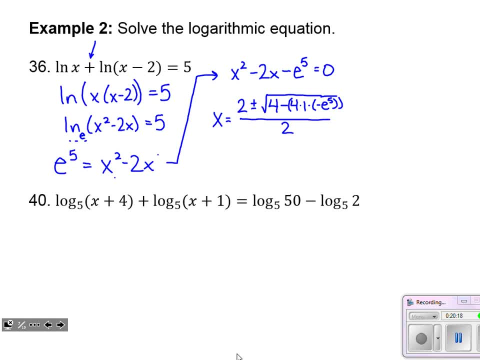 And if you've been following along, in our calculator tips and tricks section we made a quadratic formula program, So I'm going to use that right now, just for sake of time and space here in these notes, to solve this Quadratic formula. my a value is 1, my b value is negative 2, c value is negative. e to the fifth. 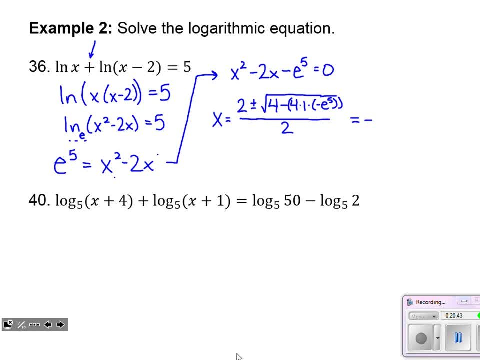 And I get two solutions. I get negative 11.22 and positive 13.22.. And let's just double check because I don't know if I can keep both of those answers if I plug them back into the original. Well, if I try and plug in negative 11.22, it's going to bother this logarithm and this one. 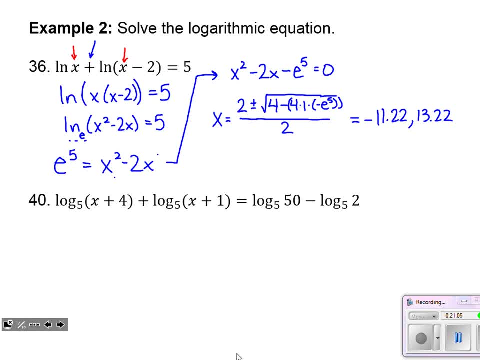 It will make both of them have negative arguments, so I cannot accept that answer. However, 13.22 will keep both of those arguments positive. That is our solution. Yikes, that had a lot. Another nice thing to consider is we did talk about- I believe it was- when we were solving polynomials. 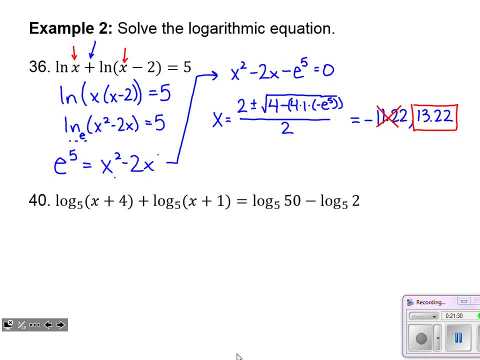 Or maybe it was with some work in chapter 5 with radicals We talked about our life hack method. Say, we get started on this problem and we get to a point where we're like, oh man, I have no idea how to solve this. 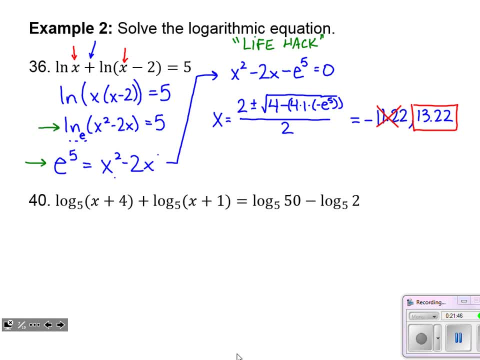 Or maybe we get to this step. I have no idea how to solve that. Well, what we could do is we could say in our calculator: y1 equals natural log x plus natural log of x minus 2. And we could set y2 equal to 5 and do calc intersect. 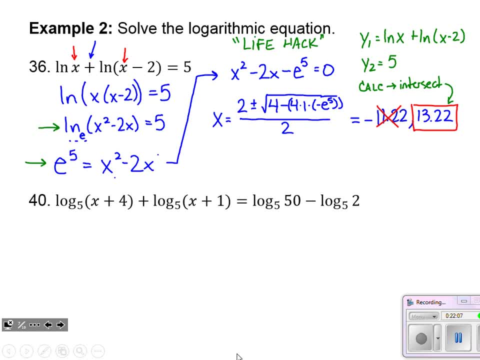 That would quickly point out this: 13.22.. That's a really nice last resort, especially like on a SAT test or in a test-taking situation, If we don't know how to do it algebraically. the calculator can provide some really good support there. 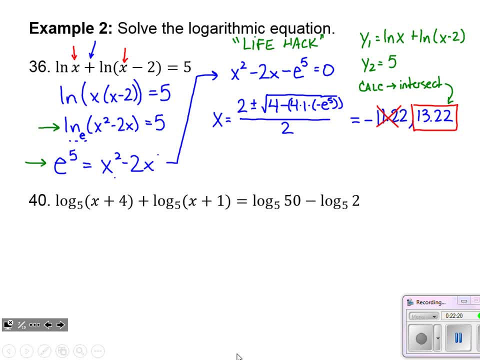 That's why I call it that. I call it the life hack, really, All right. problem number 40. Here we've got all terms that are logarithms. So I'm thinking: smash, smash, drop the logs. How would I combine these logs on the left? 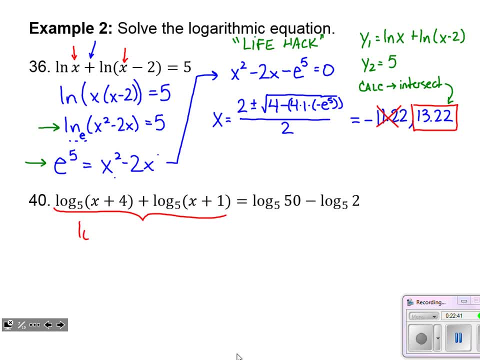 Well, they're both log base 5 and they are added together, So that's the same as one log base 5 with those multiplied together, those arguments multiplied together inside, And to multiply I would take a binomial times, a binomial. 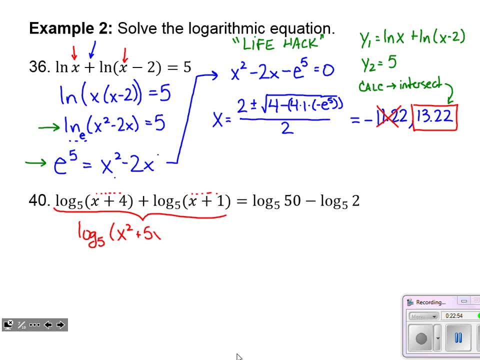 I've got to FOIL those, So I'm going to save a little bit of time by FOILing those immediately On the right-hand side to smash these two together. I know that's the same as one log base 5.. 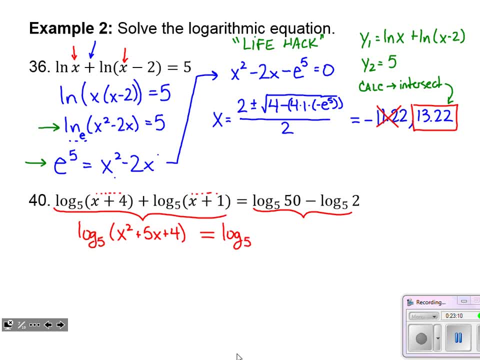 And since those logs are subtracted, it's division in the arguments 50 minus 2, or sorry, 50 divided by 2 inside would be 25.. All right, look at the condensing that we've done. Now I've got one log base. 5 equals another log base 5.. 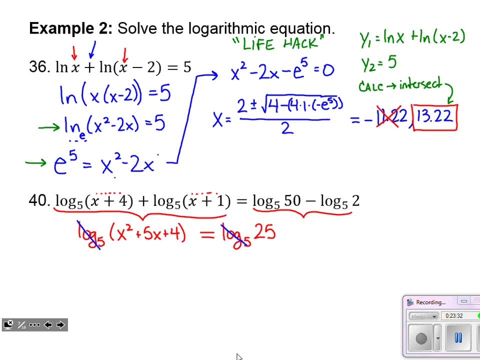 I can drop the logarithms out of it, because if they're going to be equal, their arguments have to match And my equation becomes: x squared plus 5x plus 4 equals 25.. Okay, we've got a trinomial again. very much the same situation we had up above. 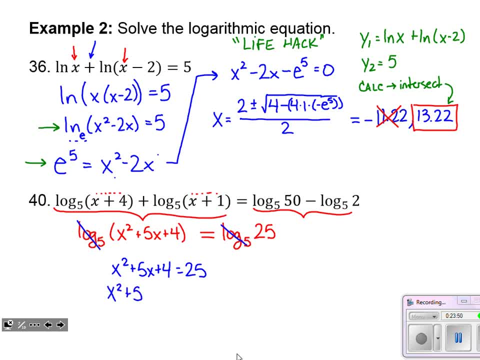 Let's get it set. Let's get that equal to 0.. Okay, and our quadratic formula says that x is going to equal opposite of b, plus or minus the square root of b squared minus 4 times a times c, all over 2 times a. 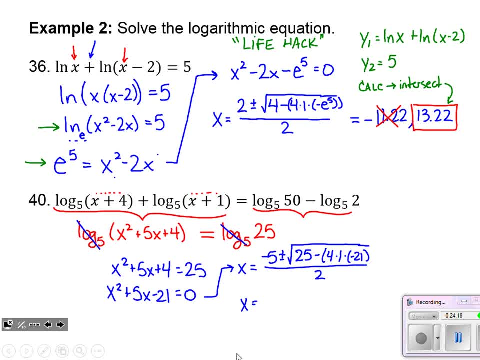 All right, and we would simplify that to get our answers According to that calculator program. let's use that again. That's why we made it in the first place. a is 1, b is 5, c is negative 21.. 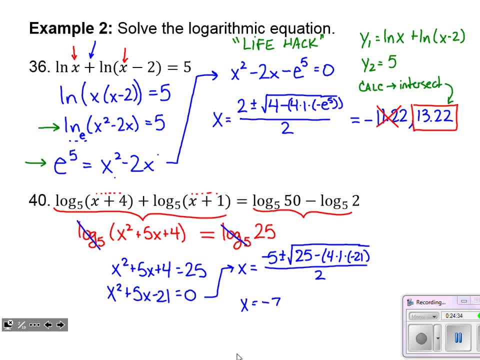 And I get negative 7.72 and 2.72.. Let's take a look at the logarithms we started with. Make sure that our solutions would not produce negative arguments in there. And that negative 7.72, man, if I plug that in here, if I added 4, it would still be negative. 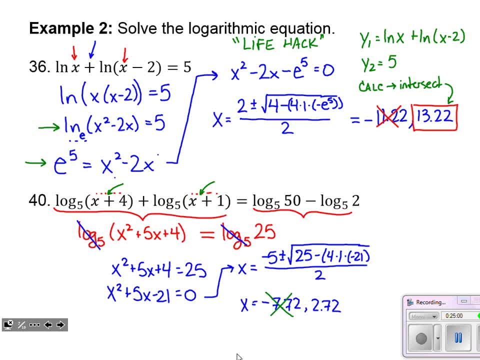 Here. if I added 1, it would still be negative, So I cannot include that. My solution is simply 2.72.. That keeps those arguments positive. That's our accepted solution. Now, keep in mind that, as you're doing this, if you're just like: wow, Mr Hartz, this lesson really went from 0 to 60 in a heartbeat. 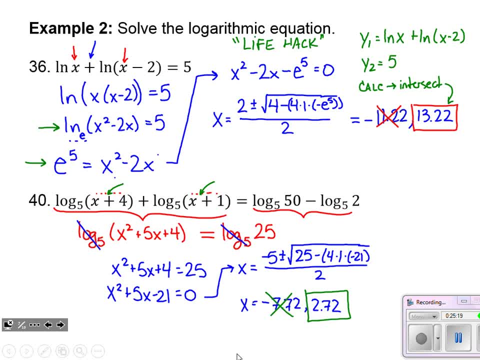 You're right, This is about as difficult a logarithmic equation problem as I could give to you, So just I hope you can take a second and appreciate the work that we're able to do on these slides with these two examples, Because we have a lot of different solving methods coming together here. 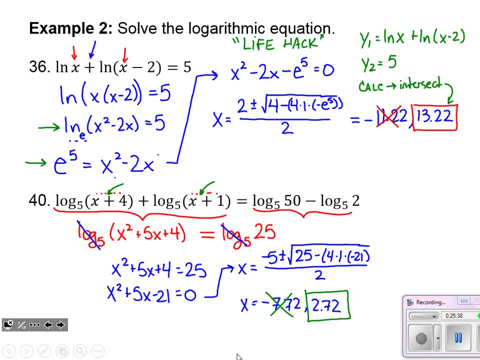 And that's the important thing to take away is look at how all this comes together so well. Learning logarithms doesn't mean we don't have to. we might not have to use quadratic formula or factoring or anything like that. It all kind of comes down to this. 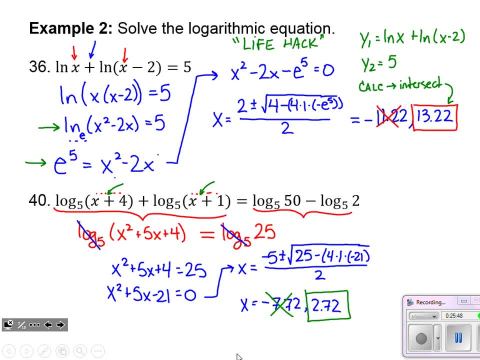 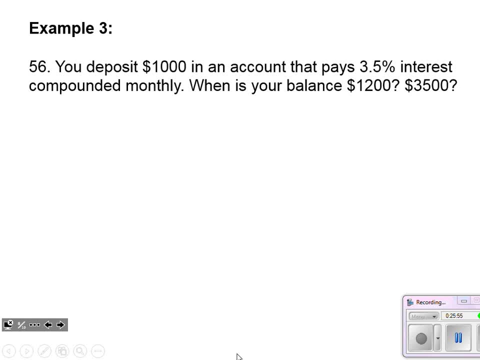 It all kind of comes together. I really like examples that do that. Our third example: You deposit $1,000 in an account that pays 3.5% interest compounded monthly. When is your account balance $1,200?? How about $3,500?? 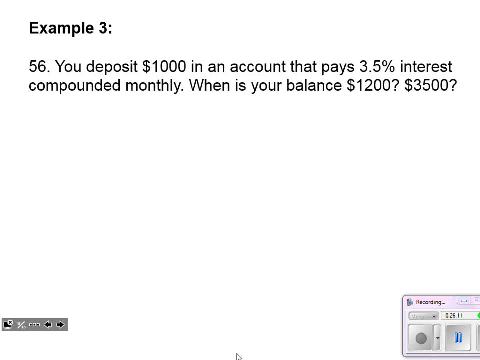 Okay. So here what we want to do is realize that we're trying to answer the when question, In other words, We're trying to find the time at which that will happen. So compounded monthly is another big giveaway. We're going to be using A equals P times 1, plus R over N to the NT power. 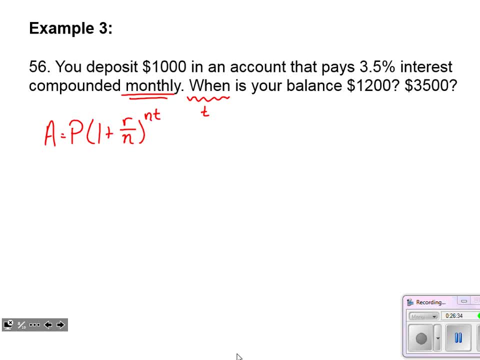 It's not continuous growth. It's happening monthly, So we need to use this formula. All right, Let's start off trying to find the $1,200 answer. The amount coming out is $1,200.. We put $1,000 in. 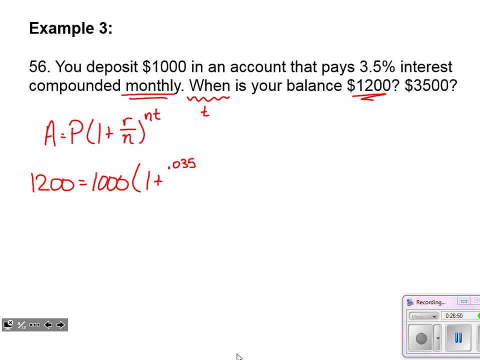 The rate is .035.. That's how I would write 3.5% as a decimal And since it's compounded monthly, that means 12 compounds per year, And I'm trying to find how many years. Well, this is a situation where we're trying to solve for a variable that is an exponent. 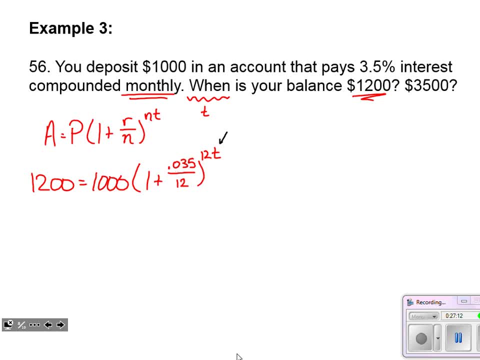 All right, We're trying to get to that T right there. First thing we want to do: isolate the exponential. Let's divide out that 1,000.. 1,200 divided by 1,000 is 6 over 5.. 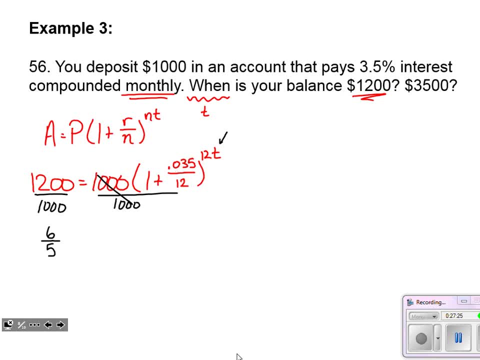 We don't really even have to simplify that. We're going to turn to our calculator eventually, All righty, That equals 1 plus .035.. I could find out what decimal this means, But again, if I'm going to type it into a calculator eventually, anyway, 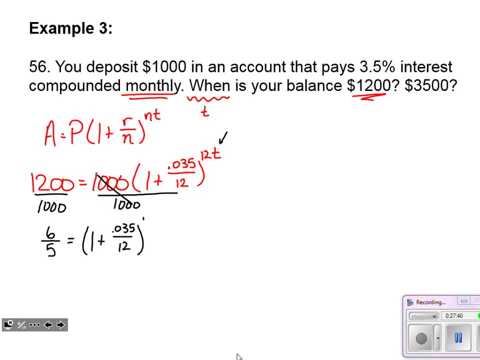 why bother going back and forth between calculator and paper? Next, what I'm going to do: I need to free that exponent, So I'm going to log both sides And technically you could use that log base method if you so chose. 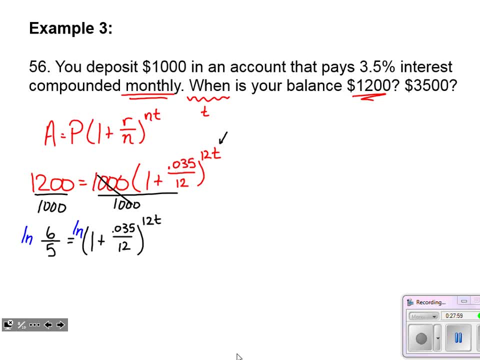 I prefer to log both sides in this situation, But it's your call That will allow us to free that 12T, that exponent. So on the left, I've got natural log of 6 over 5.. On the right, I've got 12T times the natural log of 6 over 5.. 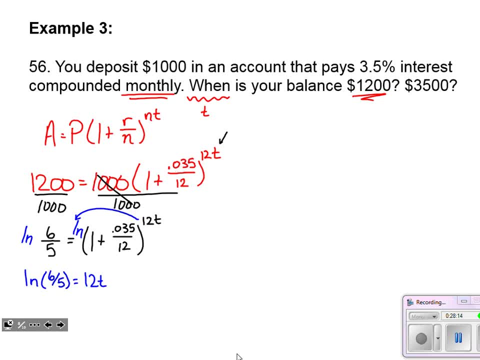 So I'm going to divide that by 12T times the natural log of 1 plus .035 over 12.. And here is the variable I'm solving, for I can divide away everything else. I can divide out the 12 natural log of 1 plus .035 over 12.. 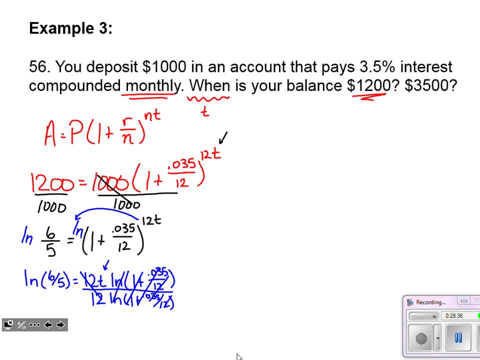 And that will cancel everything out except for the T on the right-hand side. OK, So now this is what I'm typing in the calculator And I haven't had to turn to the calculator yet in the problem. So as long as I'm careful with grouping, 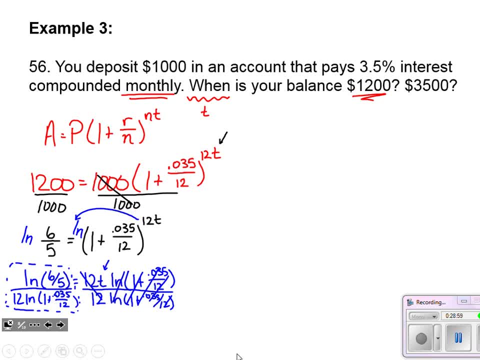 I haven't rounded anything that could change my answer And I haven't potentially miscopied something. if I typed something into the calculator early. When I type in that work that's in blue over there, I get an answer of 5.25.. 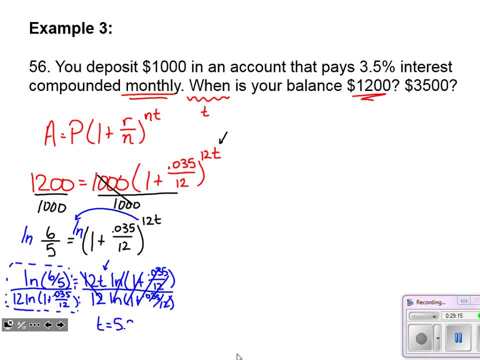 So that's 2.17.. And that is a number of years. All right. Now, with your newer calculator, it's probably storing all of that work in it, which is really really nice. because second, they ask us: 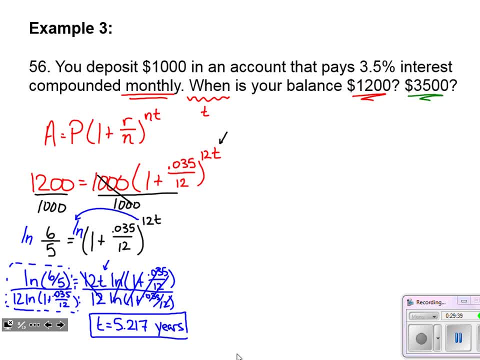 how long does it take to get to 3,500?? Well, all we're doing is changing this value right here from 1,200 to 3,500.. So I'm going to go through the exact same math, except it's going to change that number. 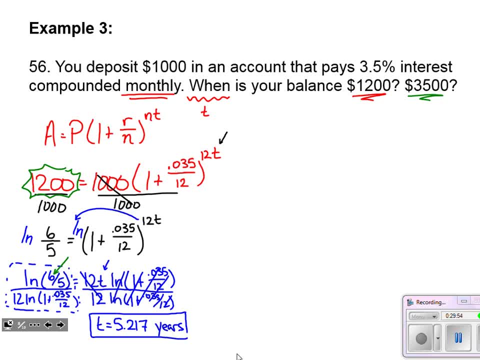 That's it. Instead of being 6 over 5, it's going to be some other number, So I'm going to spare you both the time and effort of writing all of this work out again The answer to our second part of this problem. 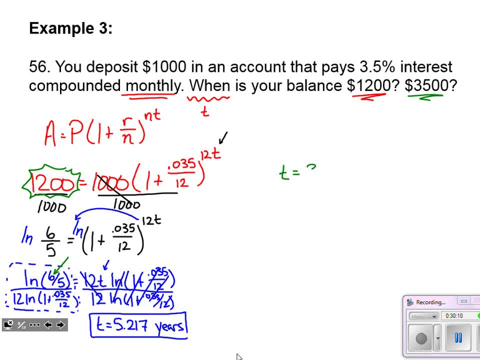 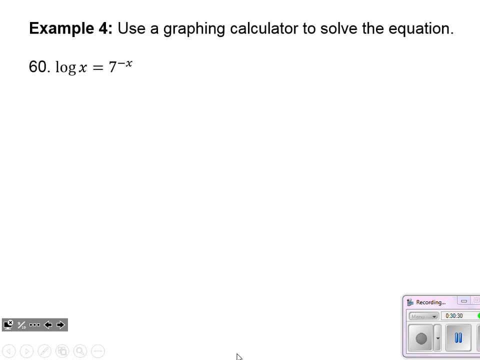 when I plug that in 35.845 years And that answer makes sense, It should take a lot longer for that account to get to 3,500, as opposed to just getting up to 1,200.. A long time with that low interest rate. 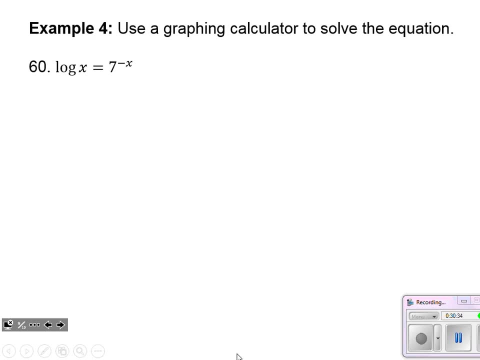 All right, And our final example here: use a graphing utility or a graphing calculator to solve this equation. And this is first and fourth, And this is first and foremost, actually only a life hack problem. You'll see that one side of this is a logarithm. 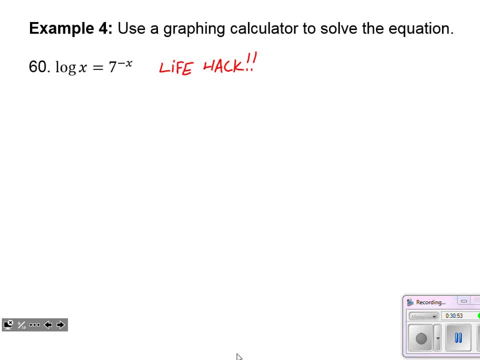 The other side is an exponential, So I can't log both sides to free the exponent. I cannot use the definition of a logarithm here, because then I will get a term that's exponential and one that's just a regular x. So really, 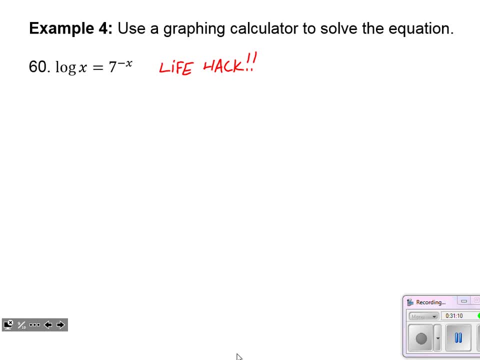 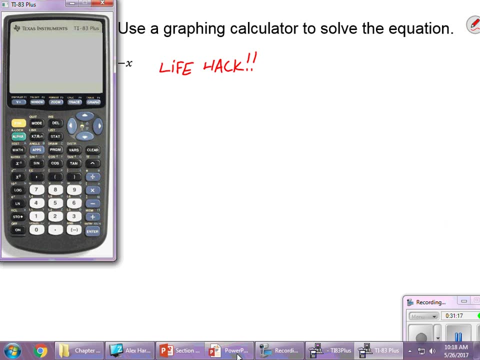 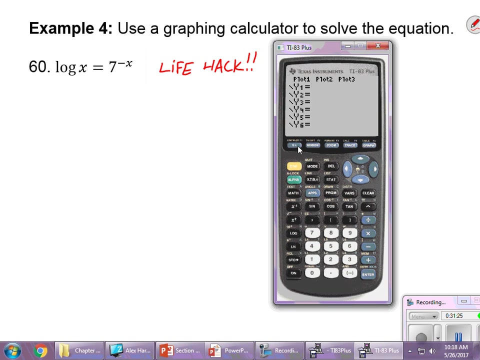 this is the only. this is a problem where the only means of solving is to use that life hack. So let me bring up a calculator here And what we're going to do is turn the calculator on, of course, In the y equals menu on the left side. 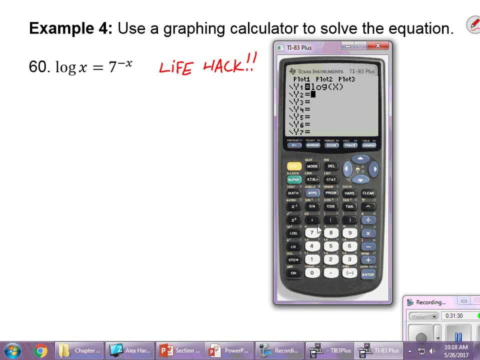 I'm typing in log x for y1.. For y2, I've got 7 to the negative x power for y2.. I'm going to graph. It sure looks like they intersect at some point there. So then what I'm going to do is I'm going to 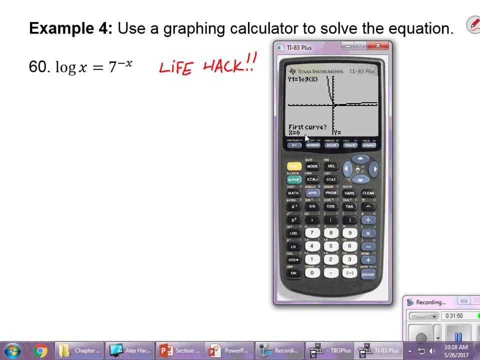 go. calc intersect The first curve. you can see nothing's showing up for y. I have to toggle and make sure that it is on that logarithmic graph. There it is. Second curve, my exponential falling to the right. It's already got that located. 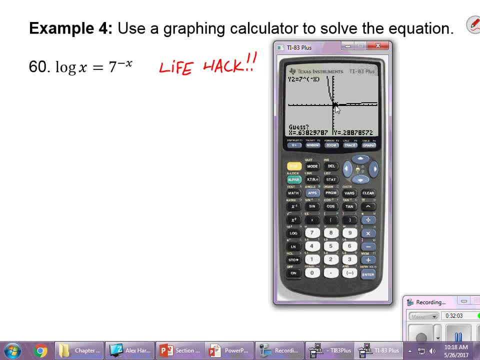 So I'll hit enter. My guess I'm pretty close to where those are intersecting, I think. So I'm going to hit enter And there I get the x value 1.233.. Let's say 1.2327..